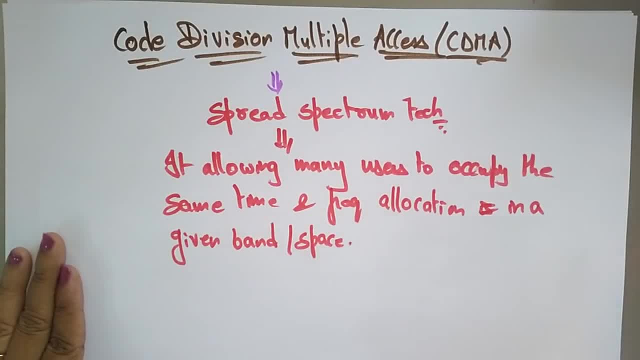 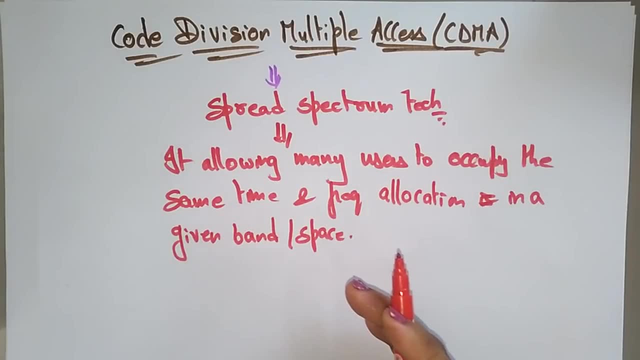 it is going to allocate uh occupy the same time and the frequency the spectral spreading of transmit transmitted signal gives to cdma its multiple access capability. so it is a form of direct sequence. it is a form of direct sequence spread spectrum, spread spectrum communication. so we call it as a cdma is a direct sequence spread spectrum communication. now. let's see what are the benefits of using this pet strength core division: multiple access. let's see the benefits. so the benefits here are: it is an outstanding voice calls, outstanding voice calls. voice and call quality will be more. quality will be more, greatest coverage for lower cost. 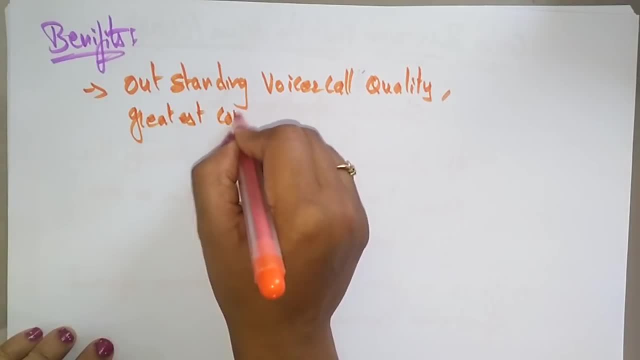 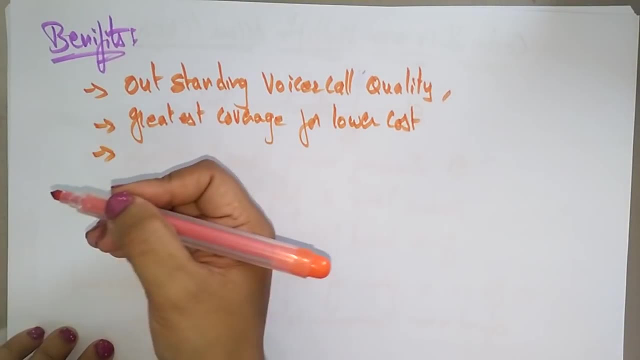 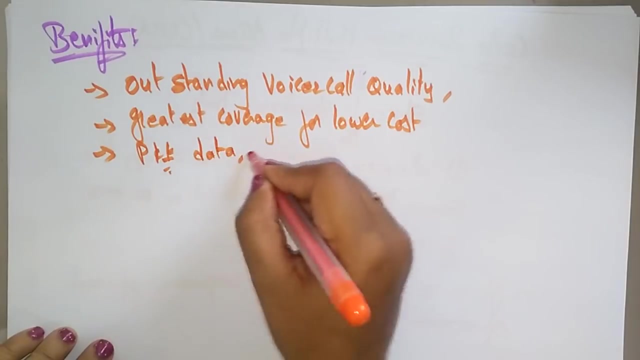 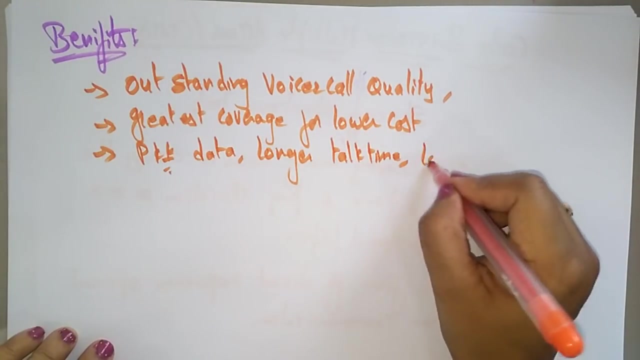 greatest coverage for lower cost. greatest coverage will be there for lower cost and packet data, longer talk time, packet data, longer talk time and long battery life, long battery life and smaller phones. greatest coverage will be there for lower cost and packet data, longer talk time, packet data, longer talk time and long battery life. long battery life and smaller phones. 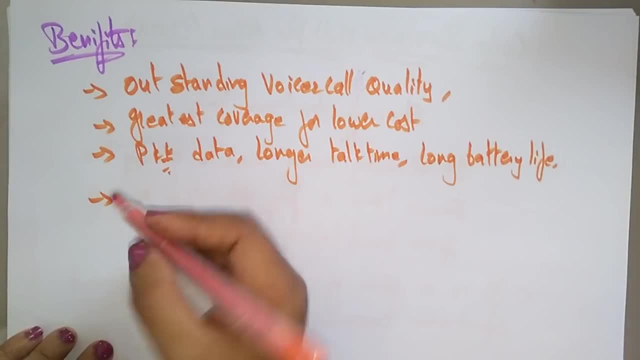 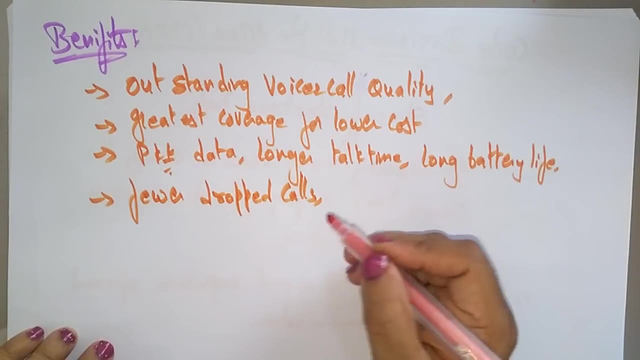 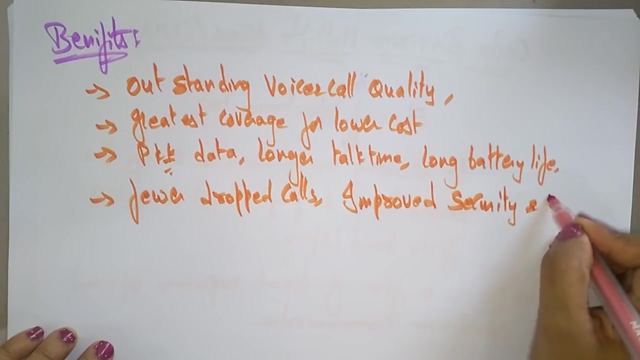 greatest coverage will be there for lower cost and packet data, longer talk time and long battery life and smaller phones. uh, still some more benefits are fewer dropped calls. fewer dropped calls- so only the less dropped calls will be there- and improved security. improved security and privacy, greater capacity. 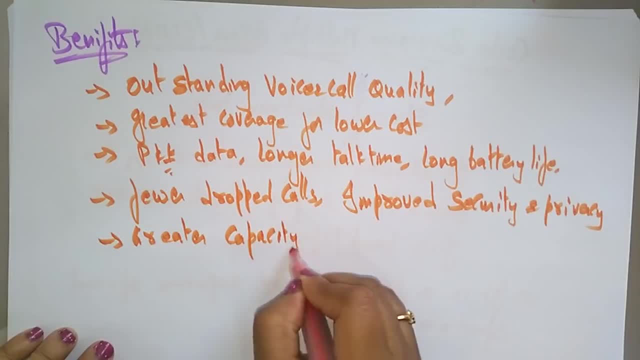 greater. it's having the greater capacity. reduced background noise- greater it's having the greater capacity. reduced background noise- greater it's having the greater capacity. reduced background noise. and interface and rapid development. so these are all the benefits of the. and interface and rapid development. so these are all the benefits of the. 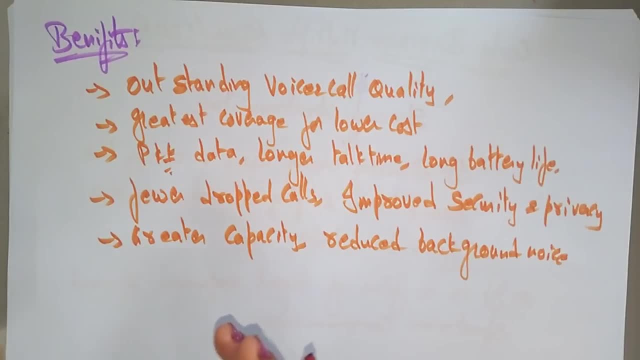 and interface and rapid development. so these are all the benefits of the cdma- the core division- multiple access. cdma- the core division- multiple access. cdma- the core division- multiple access. so with the help of if you use a cdma, you, so with the help of if you use a cdma, you. 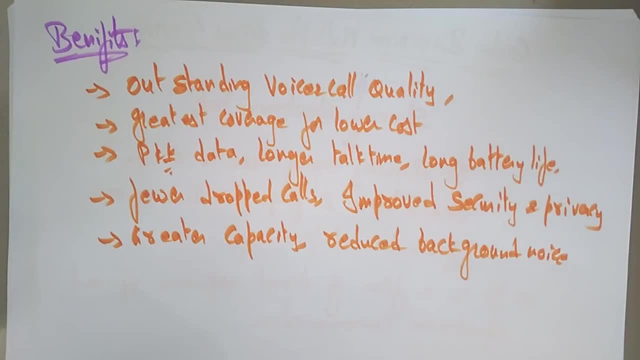 so, with the help of, if you use a cdma, you will get, will get, will get uh, the voice and the call quality is uh, the voice and the call quality is uh, the voice and the call quality is more and it covers the large coverage area more and it covers the large coverage area. 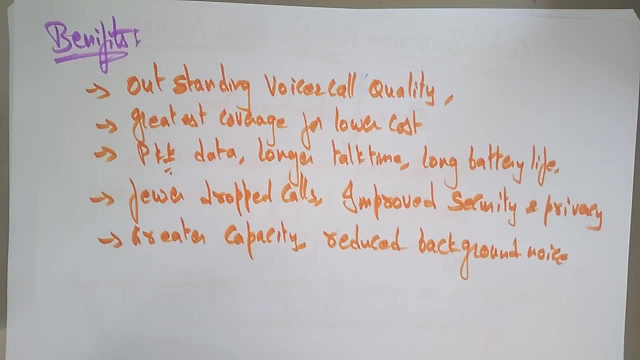 more, and it covers the large coverage area for the lowest rate, for the lowest rate, for the lowest rate. and here the battery life is long and it, and here the battery life is long and it, and here the battery life is long and it only drops. only fewer calls will be. 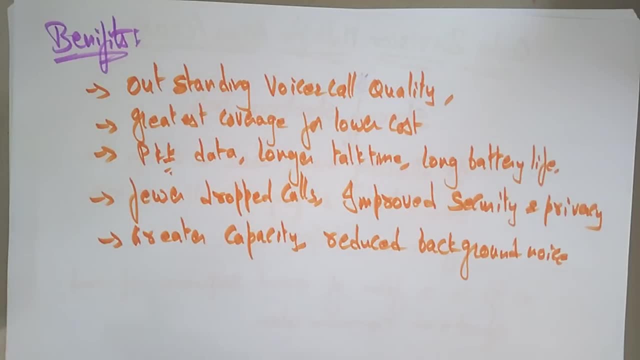 only drops. only fewer calls will be only drops. only fewer calls will be dropped. it improves the security as well dropped. it improves the security as well. dropped. it improves the security as well as a privacy. it's having the greater as a privacy, it's having the greater. 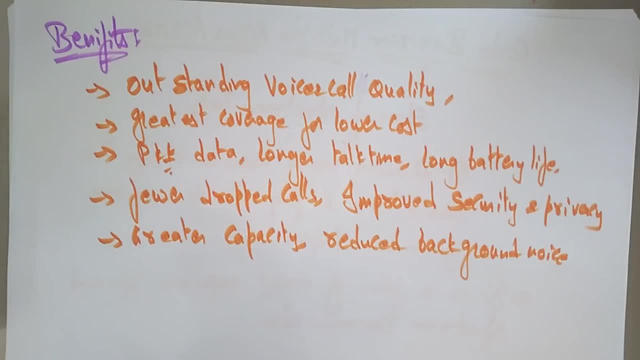 as a privacy. it's having the greater capacity and reduce the background capacity and reduce the background capacity and reduce the background noises and it also used for the rapid it noises and it also used for the rapid it noises and it also used for the rapid. it provides a feature for rapid development. 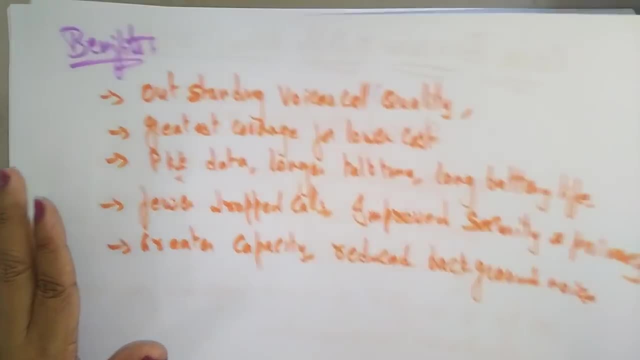 provides a feature for rapid development, provides a feature for rapid development. so these are the benefits of the code. so these are the benefits of the code. so these are the benefits of the code: division, multiple access. let me show you division, multiple access. let me show you division, multiple access. let me show you the architecture. 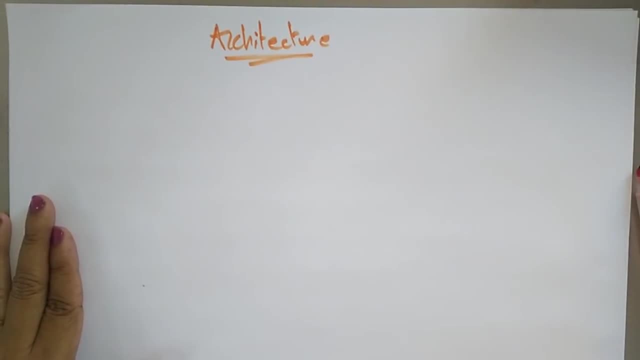 so actually the gsm gprs, all these. so actually the gsm gprs, all these, so actually the gsm gprs, all these architectures will be look, architectures will be. look, architectures will be look samey. only the difference here is they samey. only the difference here is they. 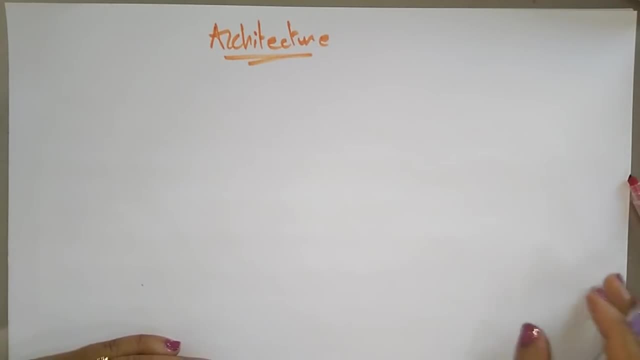 samey, only the difference here is they are using some more features, like some are using some more features, like some are using some more features, like some of extra supporting nodes will be used, of extra supporting nodes will be used, of extra supporting nodes will be used. so let's take the mobile station. 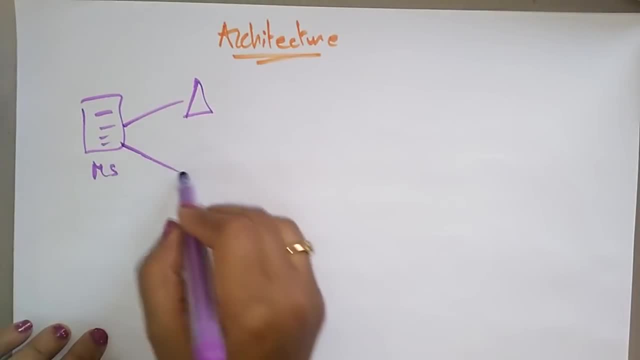 so let's take the mobile station. so let's take the mobile station. this is a let's take. this is a mobile. this is a let's take. this is a mobile. this is a let's take. this is a mobile station. the mobile stations are connected. station. the mobile stations are connected. 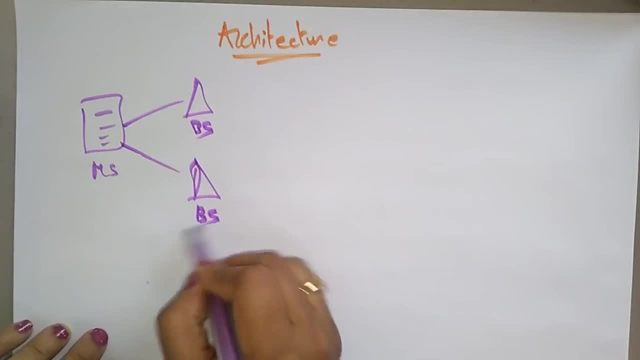 station. the mobile stations are connected to the base stations, to the base stations, to the base stations. okay, so these base stations, uh, or okay, so these base stations, uh or okay, so these base stations, uh, or monitored by the base station controller, monitored by the base station controller. 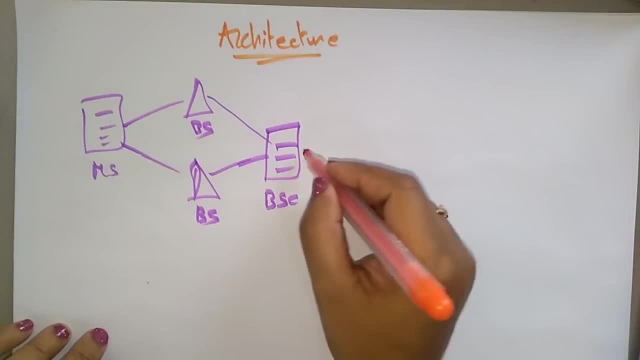 monitored by the base station controller. okay, so here in the base station. okay, so here in the base station. okay, so here in the base station controller. uh, we are, they are providing controller. uh, we are, they are providing controller. uh, we are, they are providing one switch, one switch. 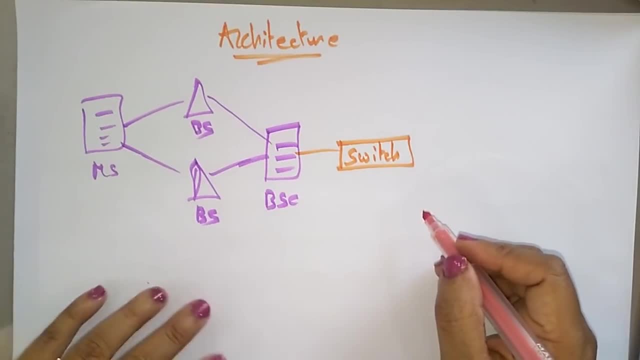 one switch. so this is an extra feature here in the. so this is an extra feature here in the. so this is an extra feature here in the. cdma a switch, cdma- a switch. cdma- a switch- switching network will be connected. so switching network will be connected. so 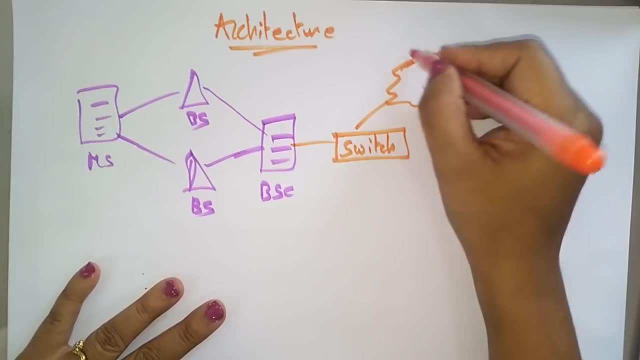 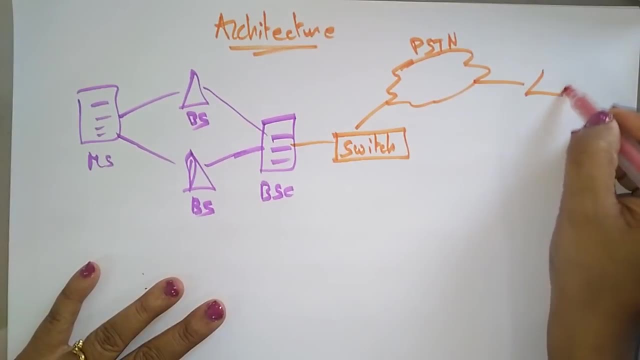 switching network will be connected. so this switching will be. this switching will be. this switching will be sent to the. this switching will be sent to the. this switching will be sent to the. that is a public wired phone network. that is a public wired phone network. that is a public wired phone network and there to your landline phones. it's a. 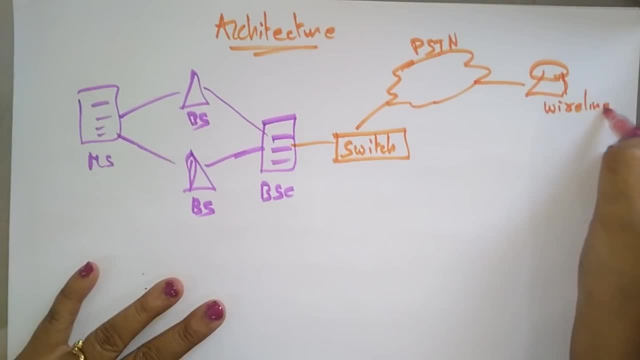 and there to your landline phones. it's a and there to your landline phones. it's a wired phone, wired phone, wired phone, wireline telephone and it also connected to this, the switch and it also connected to this. the switch and it also connected to this. the switch can also connect it to this. 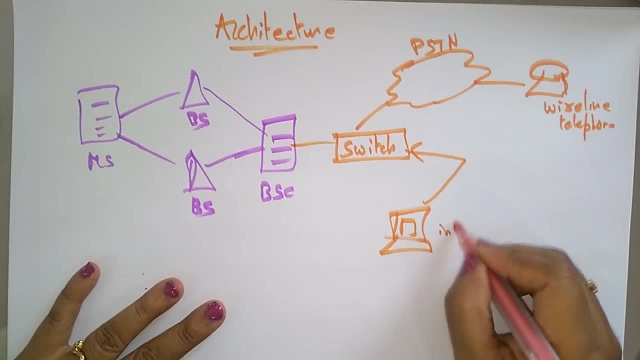 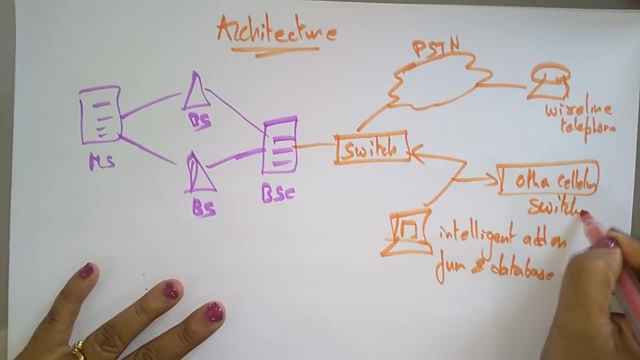 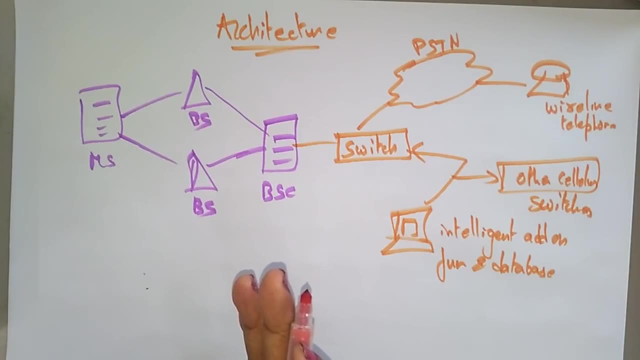 okay, and also it connects to other other cellular switches, also cellular switches, also cellular switches also. so here in this gdma- uh, you don't have so here in this gdma, uh, you don't have. so here in this gdma- uh, you don't have the uh that. 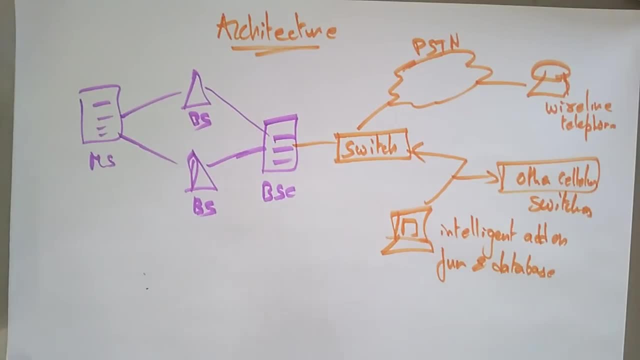 the uh, that the uh, that gateway nodes, gateway supporting nodes and gateway nodes, gateway supporting nodes and gateway nodes, gateway supporting nodes and the servicing nodes, whereas in the gprs the servicing nodes, whereas in the gprs the servicing nodes, whereas in the gprs, but in the cdma technology you are having 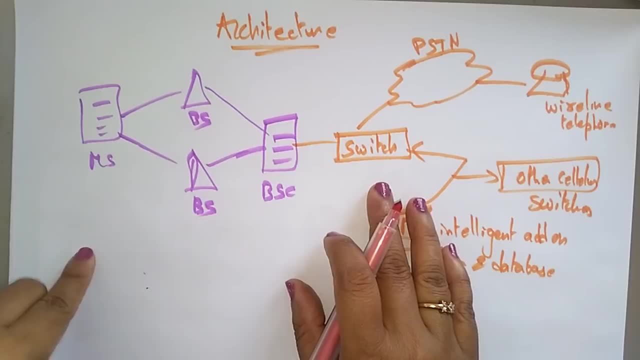 but in the cdma technology you are having, but in the cdma technology you are having the switching technology, because this is the switching technology, because this is the switching technology, because this is a spread spectrum, we call it as a spread, a spread spectrum, we call it as a spread. 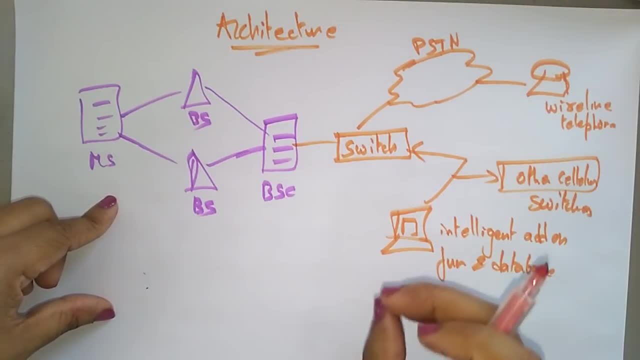 a spread spectrum. we call it as a spread spectrum, the spectral spreading of spectrum. the spectral spreading of spectrum: the spectral spreading of transmitting of a signals given to cdm. transmitting of a signals given to cdm. transmitting of a signals given to cdm. it's multiple access capability. it is 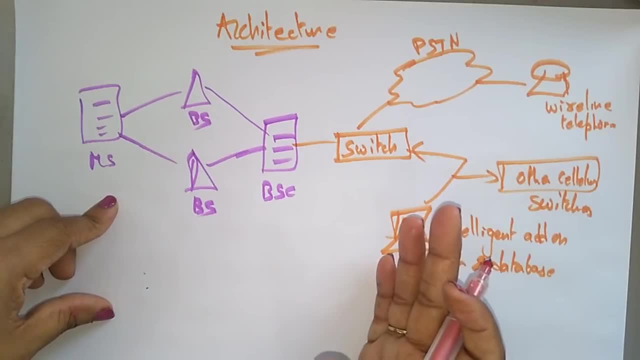 it's multiple access capability. it is, it's multiple access capability. it is multiple because of this switching multiple. because of this switching multiple, because of this switching technology, it is technology, it is technology. it is distributing to all means, allowing many distributing to all means, allowing many distributing to all means, allowing many users to occupy the same time. and users to occupy the same time and users to occupy the same time and frequency allocation in a given space, frequency allocation in a given space, frequency allocation in a given space, so it is a form of direct sequence. so it is a form of direct sequence. so it is a form of direct sequence, spread spectrum communication. 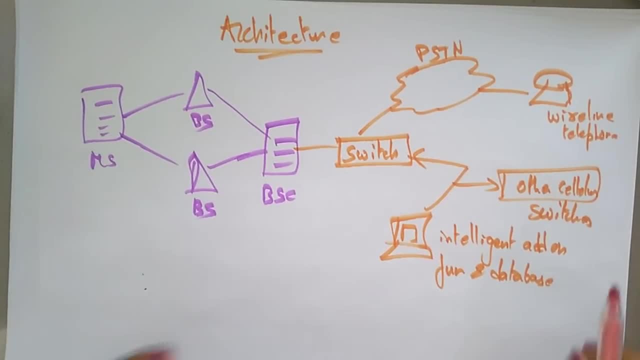 spread spectrum communication. spread spectrum communication. so cdma is different than those, so cdma is different than those, so cdma is different than those traditional ways and it does not traditional ways and it does not traditional ways and it does not allow allocate frequency or time in. 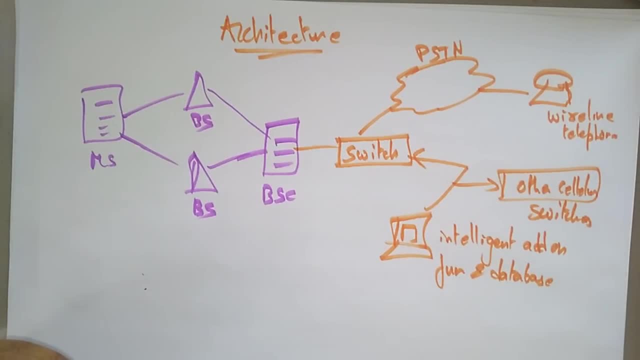 allow allocate frequency or time in. allow allocate frequency or time in users or slots. okay, you the thing you users or slots. okay, you the thing you users or slots. okay, you the thing you have to remember that it does not have to remember, that it does not have to remember that it does not allocate frequency or time in user slots. allocate frequency or time in user slots. allocate frequency or time in user slots, but it allocates both to all users. but it allocates both to all users. but it allocates both to all users simultaneously at right slots. so simultaneously at right slots, so simultaneously at right slots. so whenever they are needed, it will. 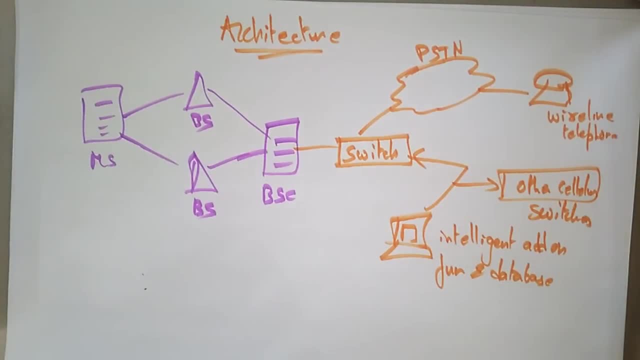 whenever they are needed, it will. whenever they are needed, it will, provided the frequency and the bandwidth. provided the frequency and the bandwidth. provided the frequency and the bandwidth. okay. so, whenever they required it. okay. so, whenever they required it, okay. so, whenever they required, it provides the time and the frequency to. 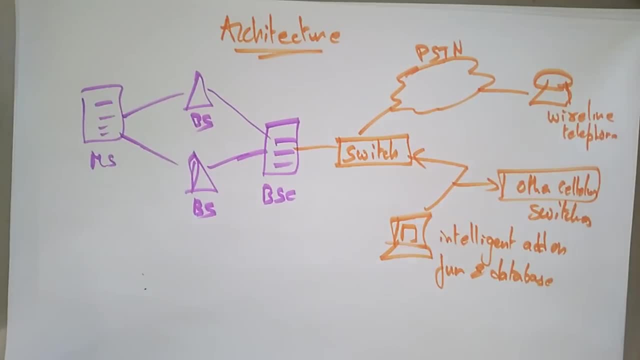 provides the time and the frequency to. provides the time and the frequency to that particular slot, that particular slot, that particular slot. so this is the features of this cdma. so this is the features of this cdma. so this is the features of this cdma. i hope you understand, thank you. i hope you understand, thank you.